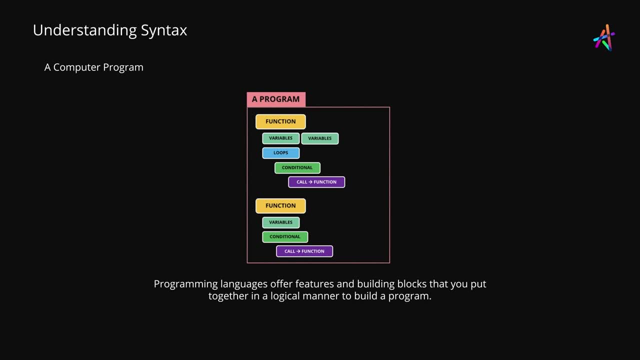 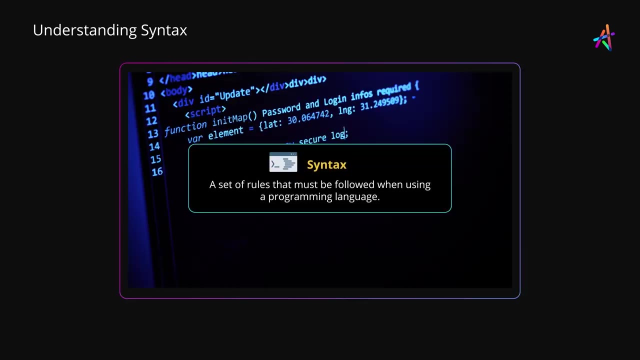 Now, every computer language is made up of building blocks that are put together to form a computer program, and we'll discuss these components or constructs later using a language called a computer program. But first let's discuss syntax. In simple words, programming languages implement a set of rules that must be followed when writing. 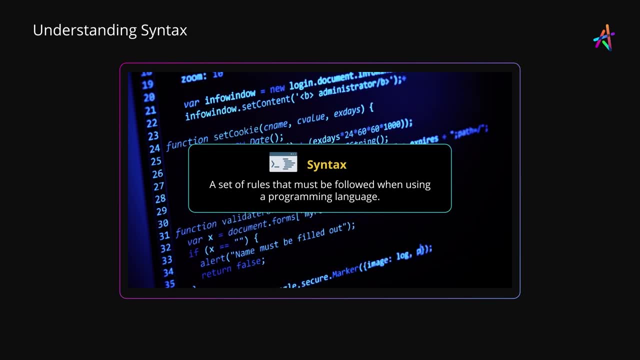 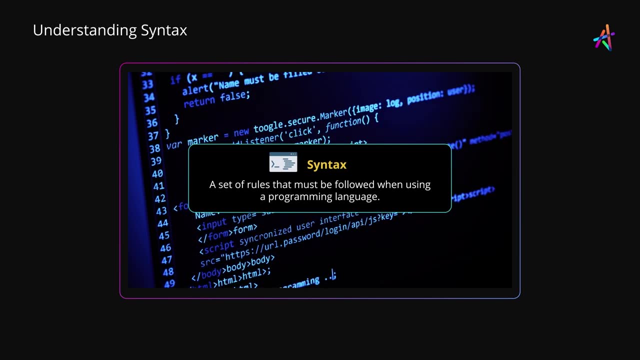 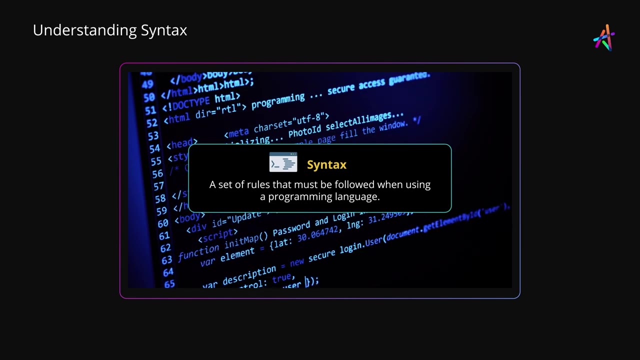 a computer program. These rules are critically important to follow for the program to work correctly and differ from language to language. Let's talk about some of these rules. However, it is not important for you to remember language-specific rules at this time. The objective is to introduce you to some of these rules so you can recognize them later. 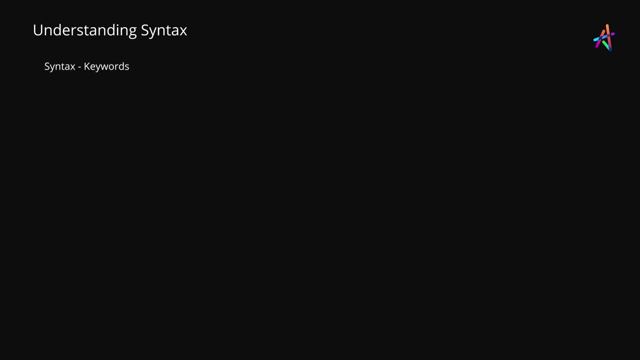 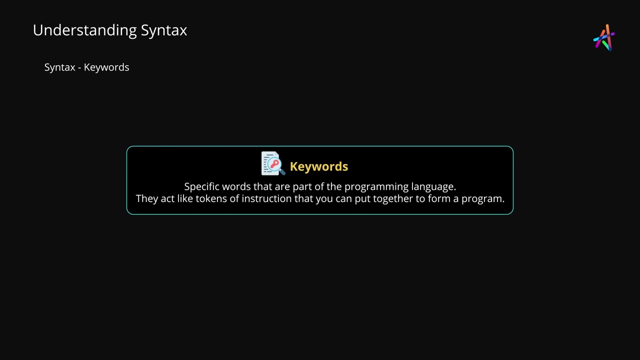 when you start writing your computer programs. Now, programming languages are made up of Keywords. These are special words which form part of the grammar of the programming language and they act like tokens of instruction that you can put together to form the logic of your program. For instance, in C++, Java, JavaScript and Python, the 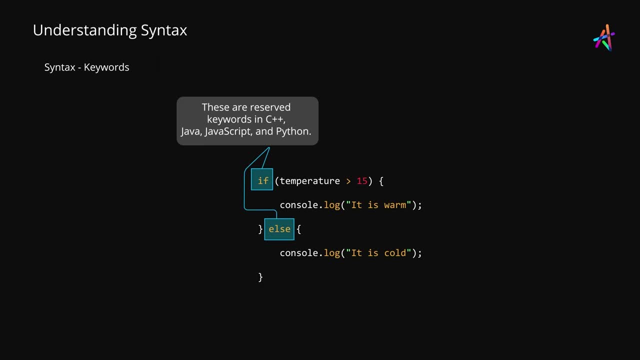 The keywords if and else are used to build a conditional statement which allows your program to take a decision based on a given set of parameters and possible values. Such keywords are reserved, which means that you cannot use them for expressing your own data in a program. 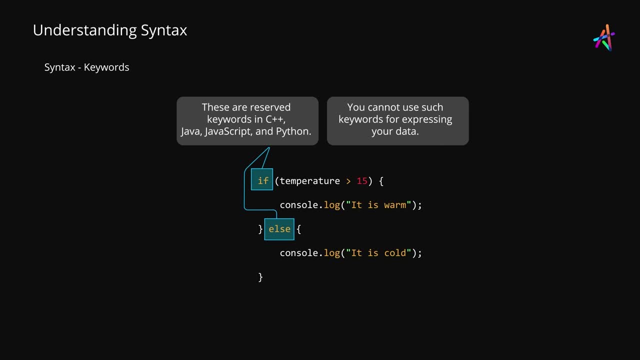 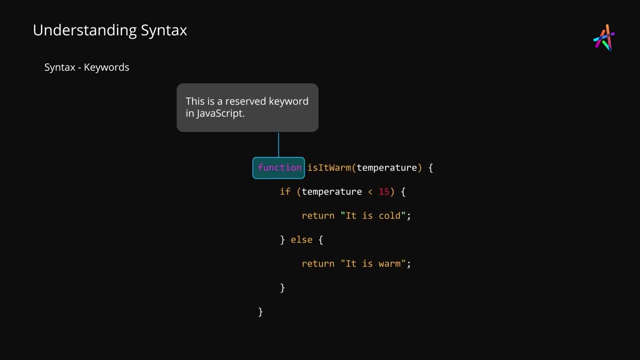 We'll understand what this means later in the course, but for now, it is important to understand that a language is made up of several reserved keywords that act like building blocks of the language and defines its grammar. In a similar way, in JavaScript, function is a keyword that. 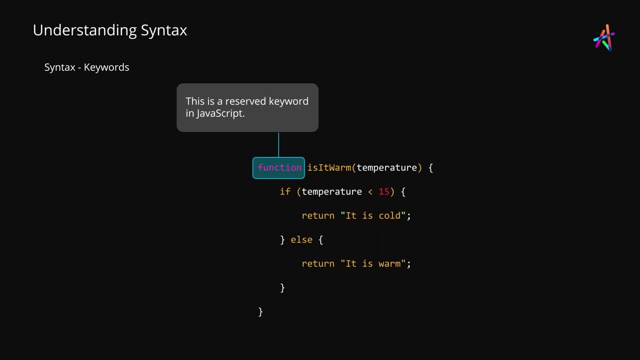 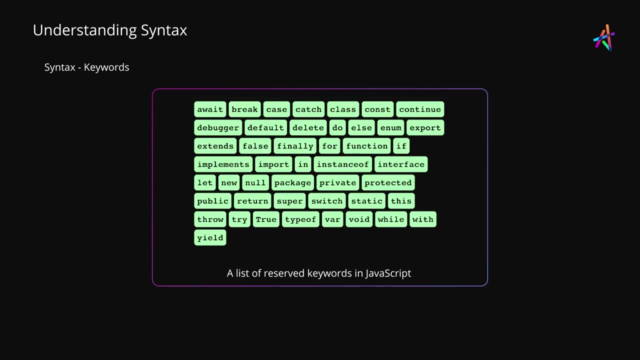 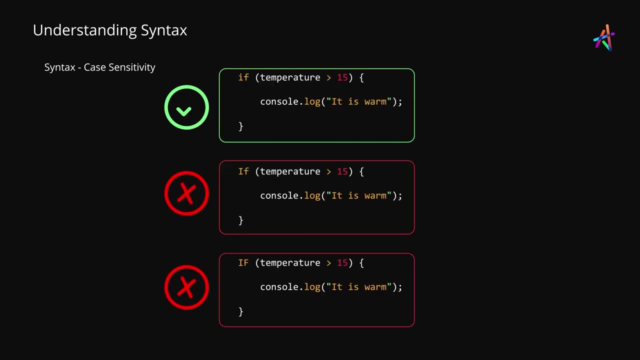 is used to build reusable blocks of code, And here's a list of reserved keywords in the JavaScript language. Now, most computer languages are also case sensitive. This means that out of these three variations of the keyword, if only the first one is correct, 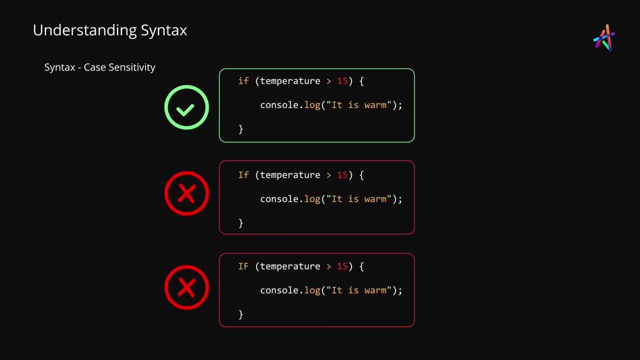 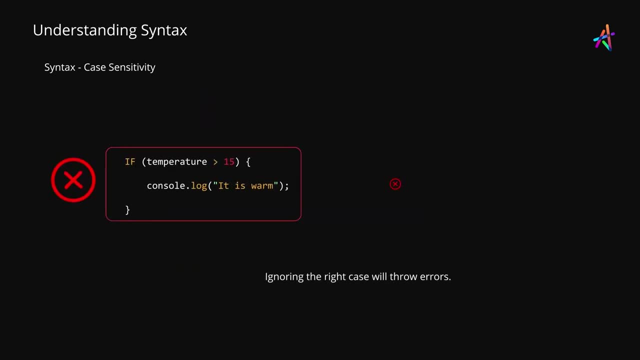 while the other two would produce an error. Case sensitivity is also one of the first few things where beginners tend to make mistakes. As with other rules, languages aren't forgiving and will raise an error if you get the case wrong Now. computer programs are like recipes. 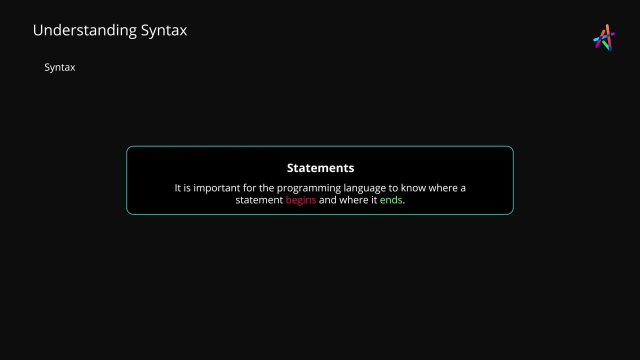 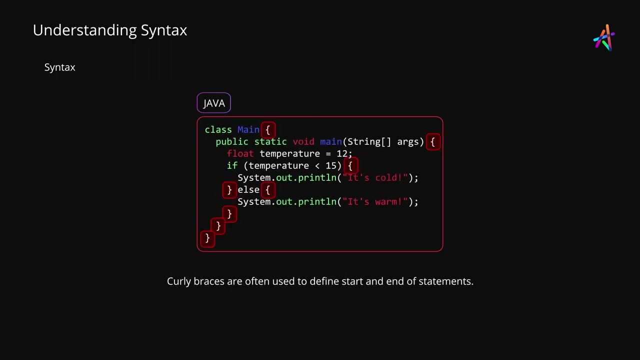 which means that, like a recipe, you have multiple instructions And it is important for the programming language to know where a statement begins, where it ends and where the next one begins. Many languages like Java, C++ or even JavaScript implement a pair of curly braces to indicate start and end of blocks of. 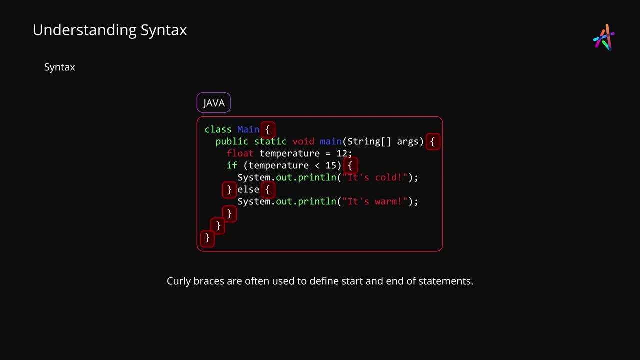 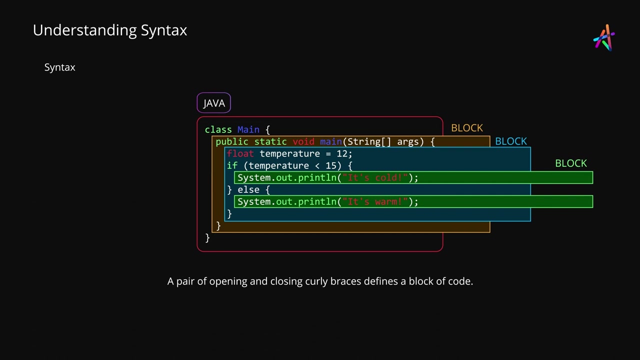 code. Here you can see a Java program with curly braces in place. An opening curly brace indicates the start of a code block, while the closing curly brace indicates the end of the block. Anything inside is part of that block. As you can also see, blocks can be nested. This helps define. 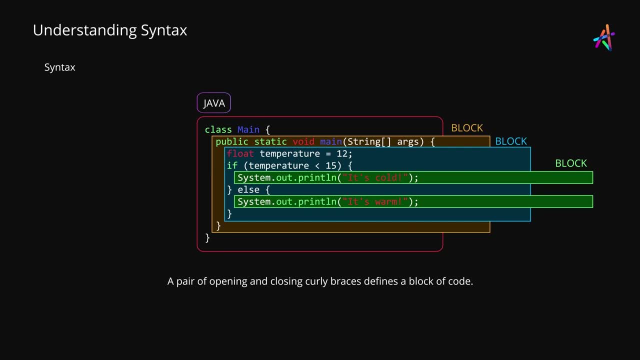 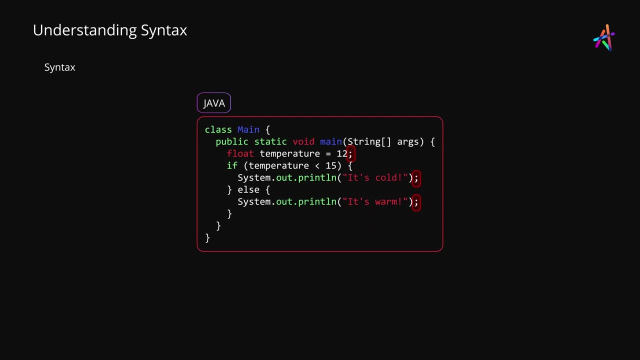 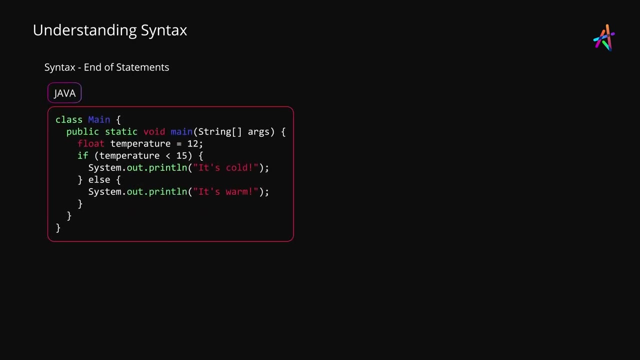 the relationship and hierarchy of statements. Another feature in many programming languages is the use of a semicolon as the last character to indicate the end of a statement. This means that this code can be written like the one on the left or even like the one on the right, and it will work because we have semicolons. 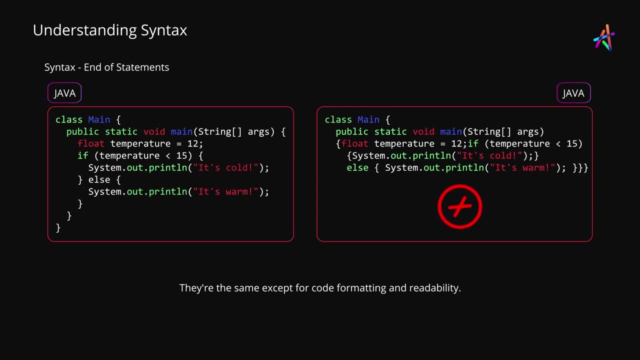 to indicate the end of statements. However, as you can see, code readability is paramount, which is why you would never write code the way it is shown on the right hand side, But the key takeaway being that the language, in this case, does not enforce formatting to create. 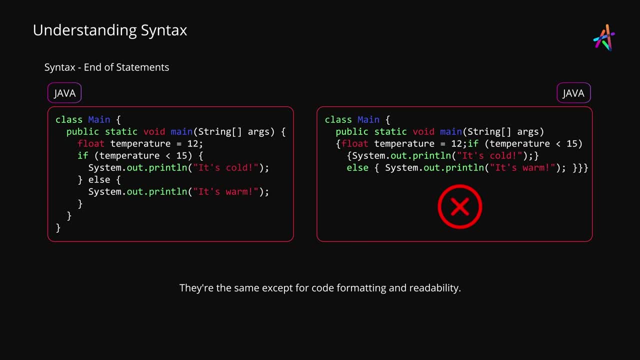 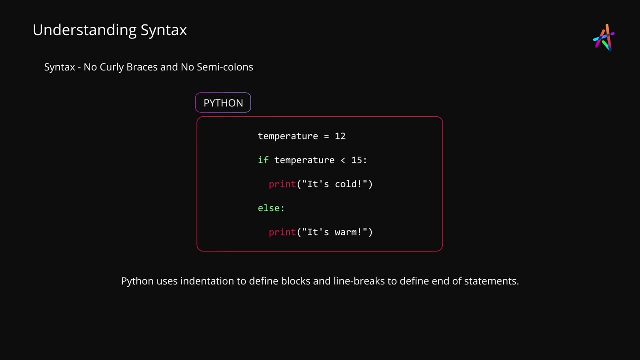 separation between statements because it recognizes start and end of code blocks and individual statements using curly braces and semicolons. This, however, may not be the case for every language. Languages like Python, for instance, do not implement curly braces or semicolons. 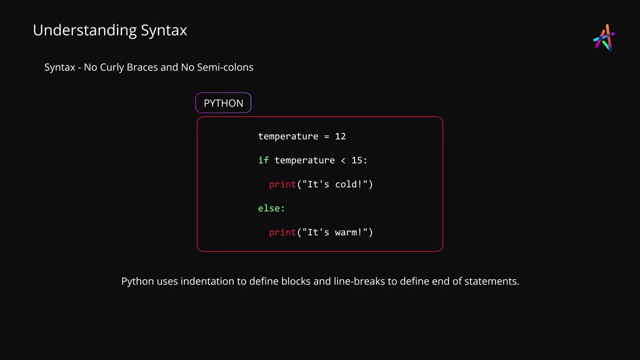 but enforce strict line breaks and indentation as a way to structure code blocks and indicate end of statements. This is why Python code looks clean and readable, not because developers love writing it this way, but because the language enforces this style, or it does. 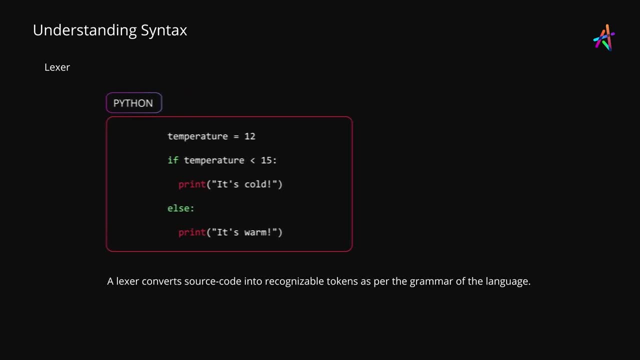 Now, the reason why these rules are in place is because programming languages include a lexer, a component which analyzes the code in a process known as lexical analysis and converts it into tokens that can be processed further. That is why lexers are also known as